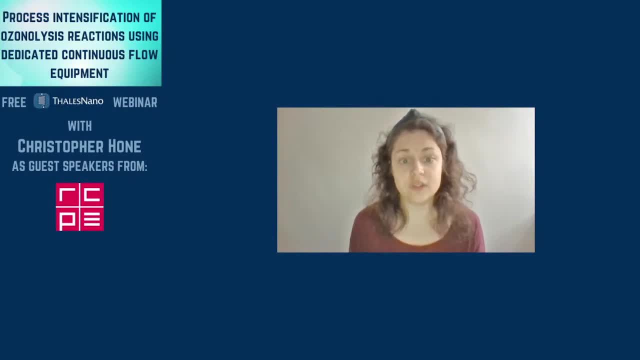 After the presentation, you will be able to ask your questions in the chat box or you can send them directly to us at askthechemist at thalesnanocom. Now let me hand you over to Christopher. Enjoy the presentation, Hello. 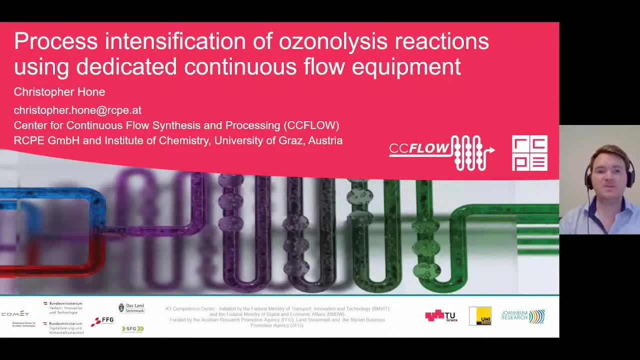 Welcome to today's webinar. I'm Christopher Horn. I'm from the Center for Continuous Flow, Synthesis and Processing, CCFlow, at the Research Center for Pharmaceutical Engineering. We're based in Graz in Austria, And today I'm going to be talking to you about the use of ozone as a reagent in organic. 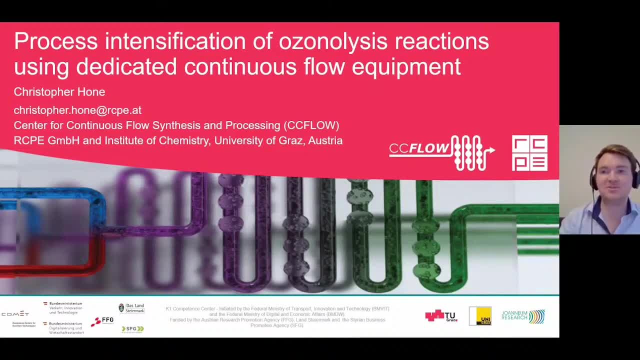 synthesis and, in particular, ozonolysis reactions, and how you can do them within continuous flow technologies. So I'll give you a general overview, to begin with, of this type of chemistry, and then I'll talk more specifically about a research case from our group. 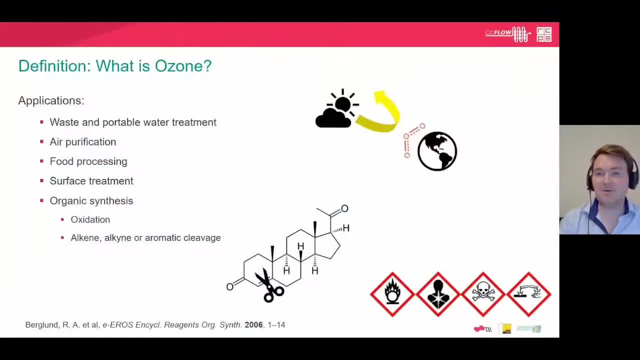 So ozone is a naturally occurring molecule. It forms from molecular oxygen within the atmosphere by the action of ultraviolet light and electrical discharges. It's very unstable, and it also has many commercial applications as well, so many of which I'm sure you're familiar with. 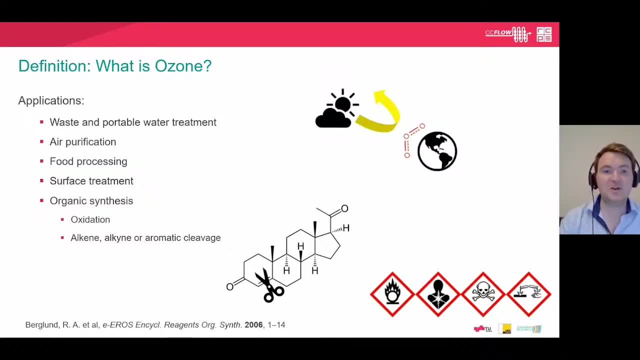 And the one that we're most familiar with is the ozone reaction. The one that we're most interested in is naturally organic synthesis, so oxidation-type chemistry and also the use of ozone for performing alkene, alkyne and aromatic cleavage-type. 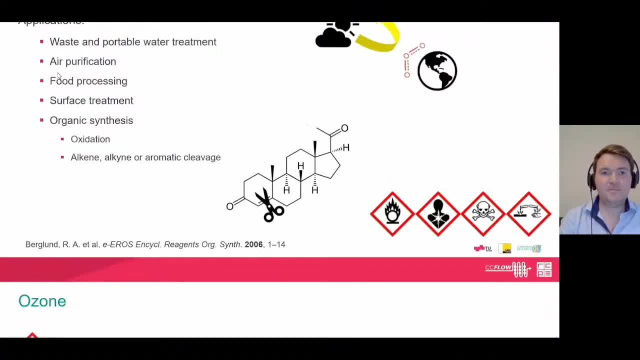 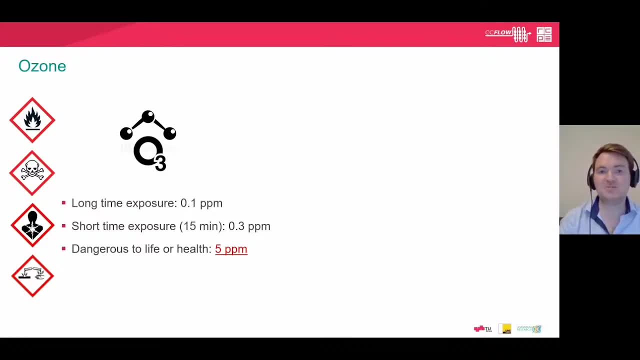 reactions. So ozone itself: it's got a bent-type structure, so it's got a similar structure to water. Ozone is a gas with a very puncture. It's got a very potent odor. It's pale blue in color, And one thing that I'm sure we all know about is it's a very toxic gas as well, so it's 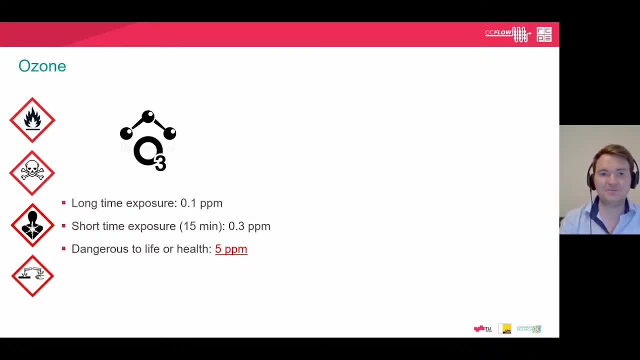 very dangerous to health, so it needs to be very carefully handled In terms of its drawbacks within batch vessels. so these are the drivers of why, then, we would want to perform this type of chemistry within continuous flow technologies. is that the accumulation of ozone within the headspace and within the liquid phase of batch reactors? 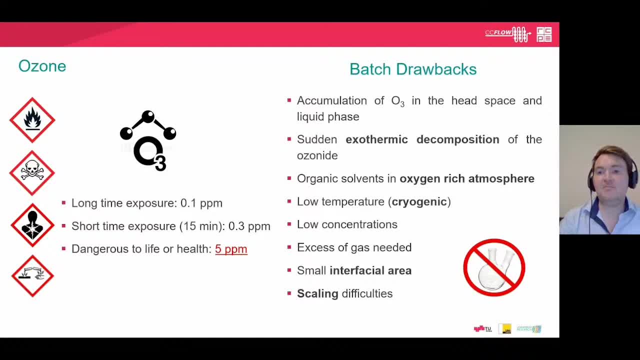 is very dangerous. We also have the ozonide intermediate that forms with this chemistry that undergoes a very exothermic decomposition, so this needs to be very carefully controlled. We are operating with organic solvents and within these systems we have very oxygen-rich. 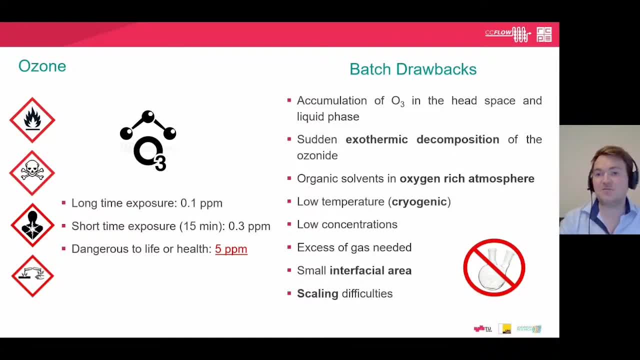 atmospheres. So there's the potential for flooding. So there's the potential for flooding. So there's the potential for flooding. So there's the potential for flammability, Because we need to carefully control the temperature. then we use cryogenic conditions which can. 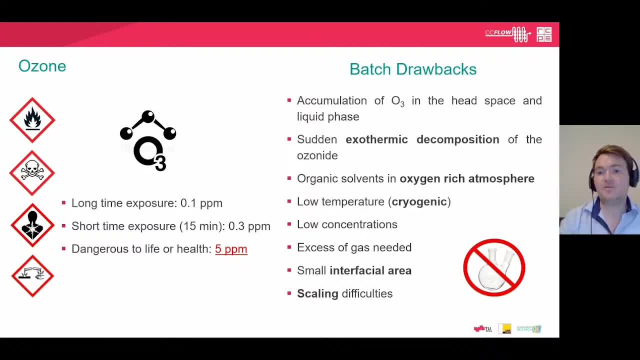 be quite challenging to handle in terms of accessing those lower temperatures, particularly at scale, Because we want to try and minimize many of the exothermic intermediates. then we operate this type of chemistry at low temperatures. These include all types of solvents that need to be processed. 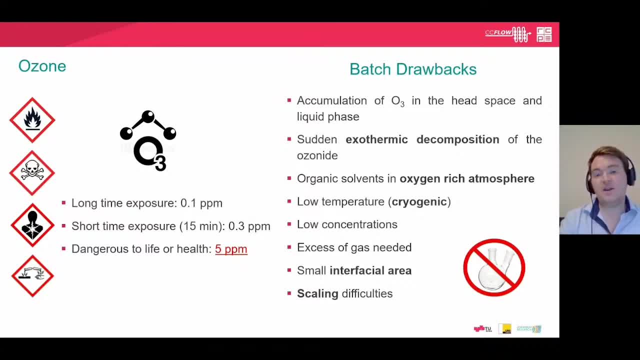 These include everything from gas, which there are no concentrations. We also need an excess of gas, So this is quite inefficient And then as we go to large scales we have quite a small interfacial area and then reactions can become mass transfer limited. 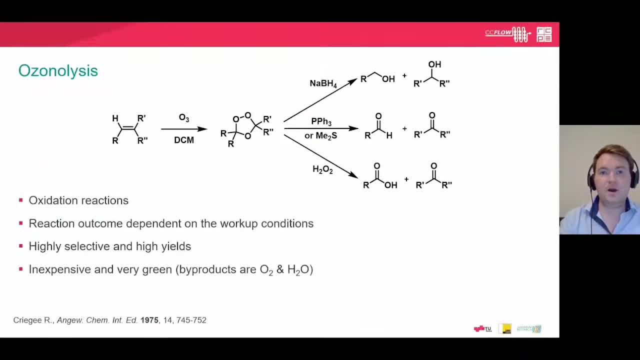 So all of these aspects then clearly lead to scaling difficulties. So the type of chemistry that you can do, So at the top we have an alkene element That's excellent, based reaction with ozone, and then the nice thing about this chemistry, depending on the 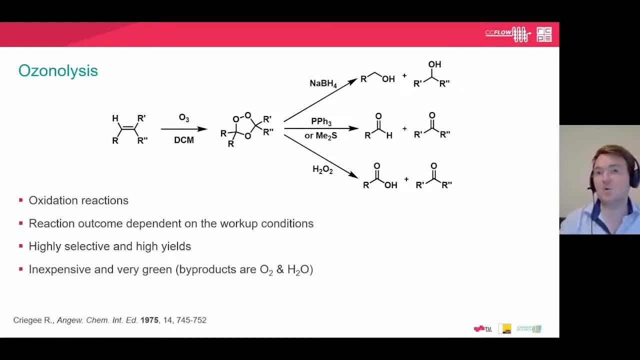 quenching reagent use. so the workup conditions. we can actually access quite a number of different products, so it gives us quite interesting molecules ranging from alcohols to ketones and aldehydes, and then also acids, and in general these reactions are quite highly selective and 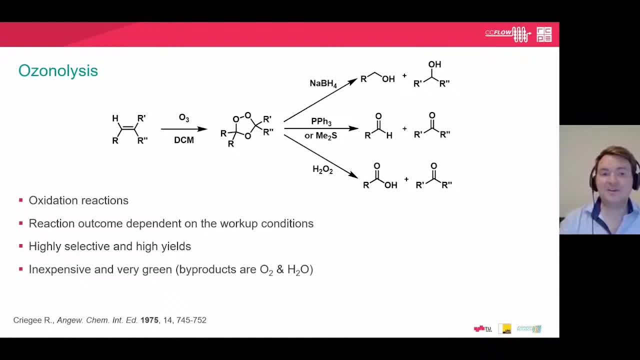 also provide high yield, and they are quite green as well. in terms of that, the only stoichiometric byproducts that we form from these reactions are oxygen and water. so there are potential benefits, even though there are limitations when it comes to handling the chemistry in terms of the safety, 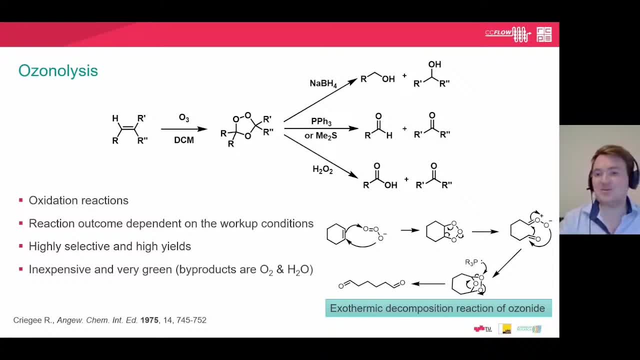 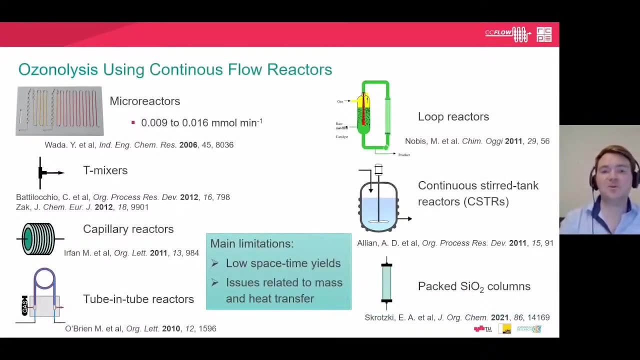 and again, this is just a mechanism to show that, from the intermediate that we observed, then this can exothermically, this decomposition of this can be quite exothermic. so just turning now to give you an overview of what's already been done within continuous flow. 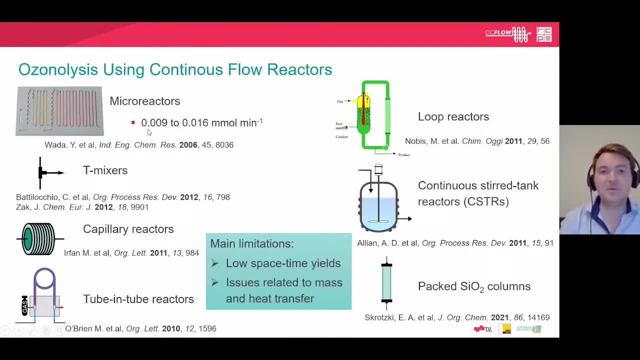 so the first example for it was from Jensen within a micro reactor back in 2006. this was sort of in this study. they basically paved the way to show that it was possible to do this. perhaps the main take-home message is that it's very difficult to achieve high throughputs within. 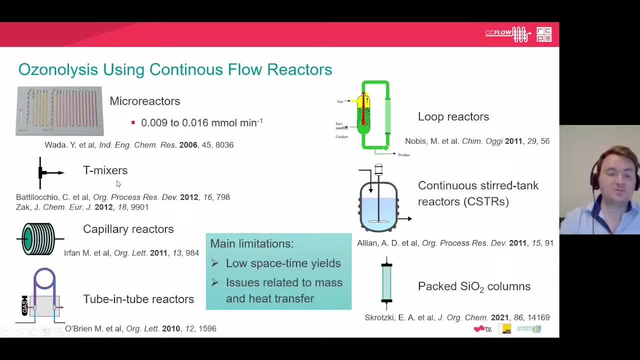 this type of system. then subsequently Stephen Lay's group looked at just using tea pieces for performing ozone analysis reactions, and this works very well because generally these reactions occur very quickly. so on the second to millisecond time scale, the problem comes is when you want to scale this chemistry up within a tea mixer. then you need larger diameters and you can. it can be hard. 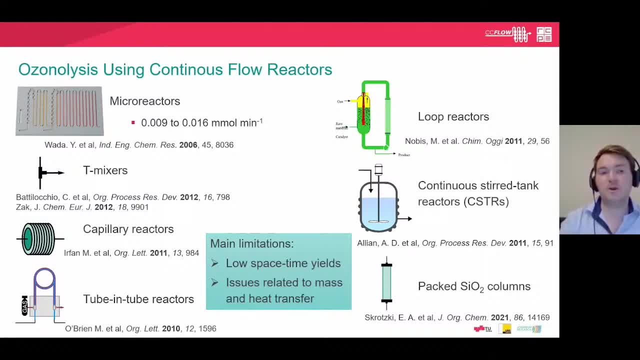 to predict how then the chemistry will perform at large scale and how do you thermally manage the system? also an earlier example from our own group: using tubular capillary type reactors to perform this chemistry. again, this has limited. this had the same limitation in terms of it was a relatively low throughput and it's very 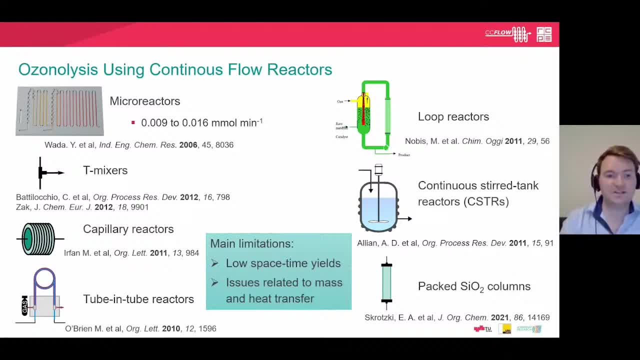 difficult to scale from this kind of reactor for a gas liquid type reaction. and then Stephen Lay's group also reported the use of ozone within tubing tube reactors. this is a very interesting approach whereby there's a tube within a tube, with the middle tube is constructed of a semi-permeable membrane which allows passage of the gas through. 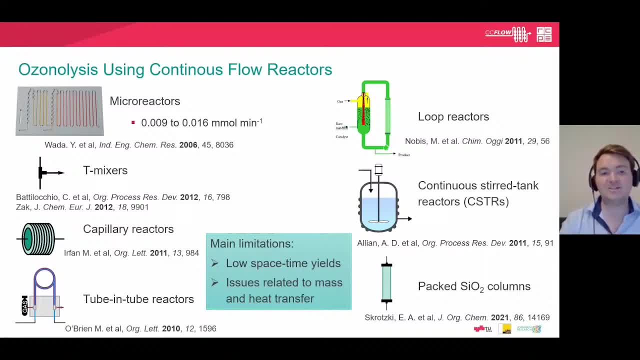 but doesn't allow passage of liquid. so it means you have your gas and yours allows the passage of ozone through, which means that then you don't have a gas liquid system within one compartment, so the the ozone is all dissolved within the liquid phase, which makes it safer to 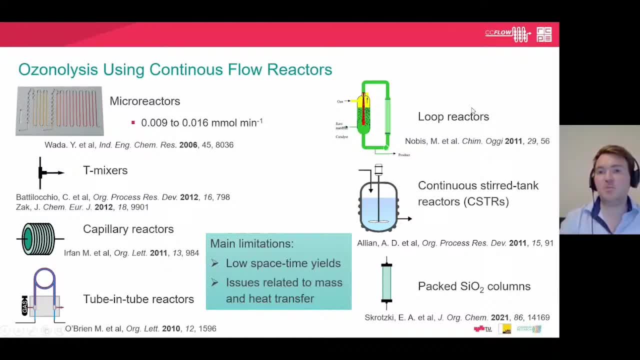 handle. also, loop reactors have been reported whereby the liquid feed is recirculated through the reactor. this can be quite useful for operation at scale. continuous stirred tank reactors, again another solution for operating at scale. the ozone needs to be carefully kept below certain levels. so this is a challenge, because a cscr in some ways has similarities to batch type reactors. 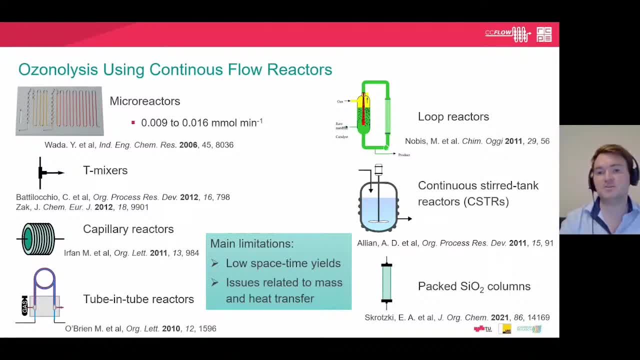 but it does give the potential for scale up by continuously throwing through through your liquid feed and then very recently um, a, a, an approach whereby silicon dioxide, um columns were used to enable a solvent-free uh synthesis without um uh for uh ozonolysis reactions. so the main limitations of this type of chemistry is that in general, you see, quite low. 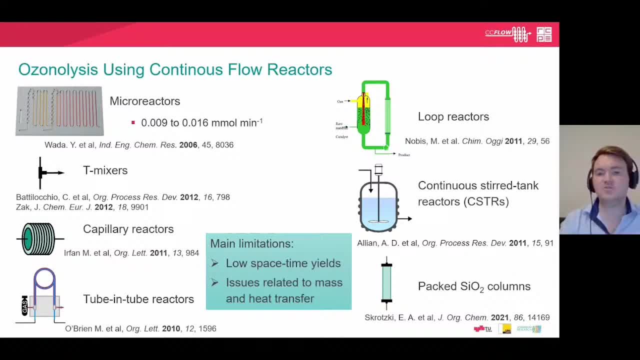 space-time yields, and there's often issues related to mass and heat transfer. so any any purchase that can try and address this um can um clearly help in terms of scalability. but these are all excellent, uh examples of um how ozone has been used as a reagent for. 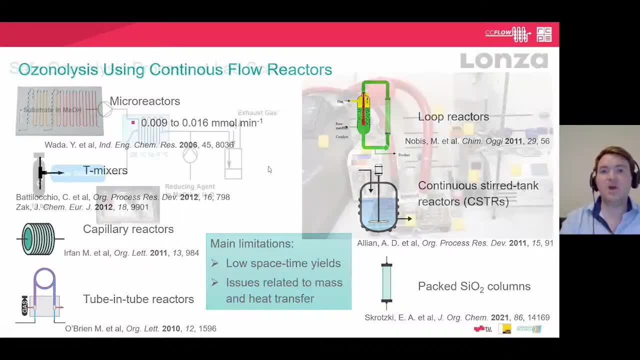 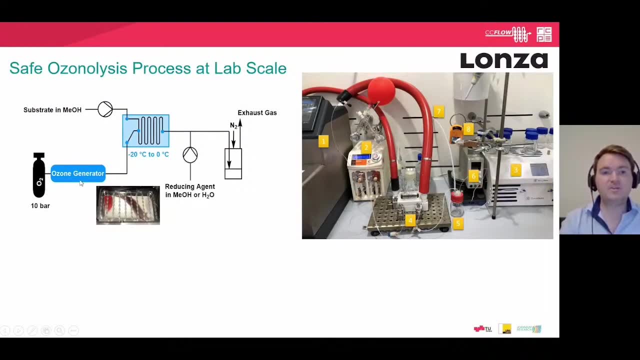 reactions within continuous flow- um. so here is our general setup in terms of we have oxygen which then passes through an ozone generator to form um ozone, and we have our liquid feed, which is introduced uh via a pump- uh- and then this flows through a um, a microreactor. so 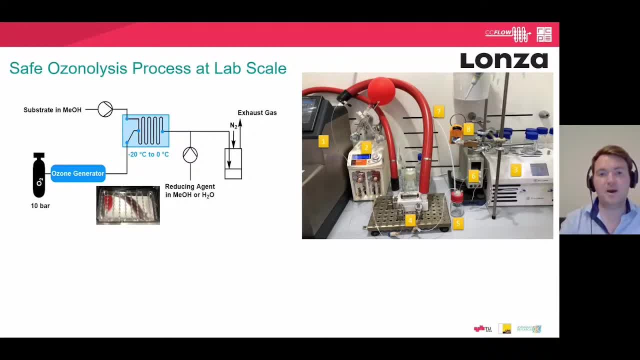 in this case the lonza flow plate manufactured from uh by airfoil, and then, at the end of the reactor, we have our quenching feed and then this flows into a vessel which has a nitrogen purge and an exhaust gas to ensure that, um, we don't have high levels of. 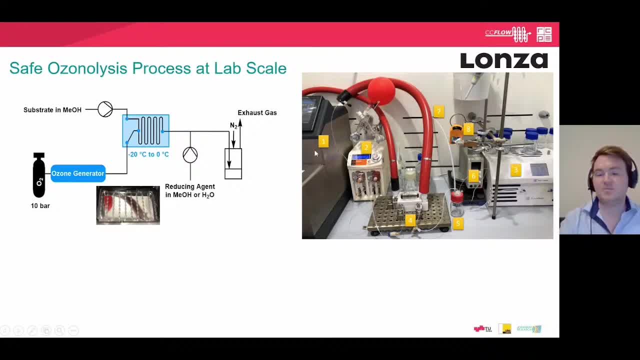 undesired gas. so on the right hand side we have the setup as a picture, in terms of having the thermostat. we have a serious syringe pump for introduction of the liquid feed, the flow plate- here we have our outlet chute. and then we have a pump for the flow plate- here we have our outlet. 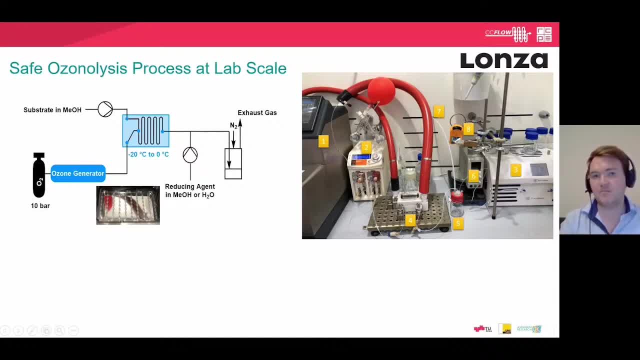 tube in here which has our vent and our um and our nitrogen purge, and then over here we have our tallies nano ozone generator. so, again, as i mentioned, an inline quench is very important to ensure that um we don't see the accumulation of um potentially um exothermic intermediates. 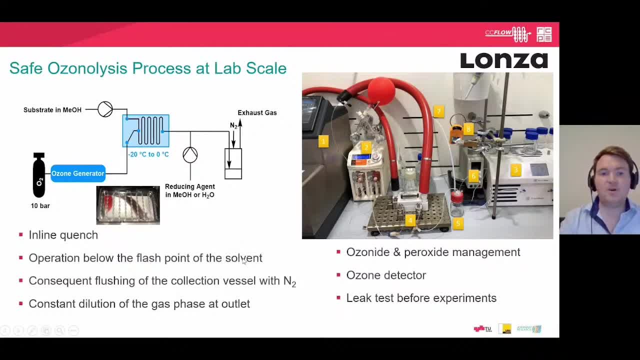 and explosive environments. we want to try to operate below the flash point of of the solvent to ensure that, uh, there's not any chance um of explosions. and then also we want to keep diluting the um outlet vessel with nitrogen gas. and then also, here you can see the ozone detector. 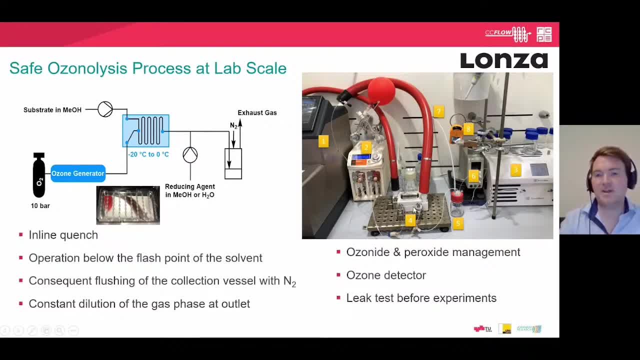 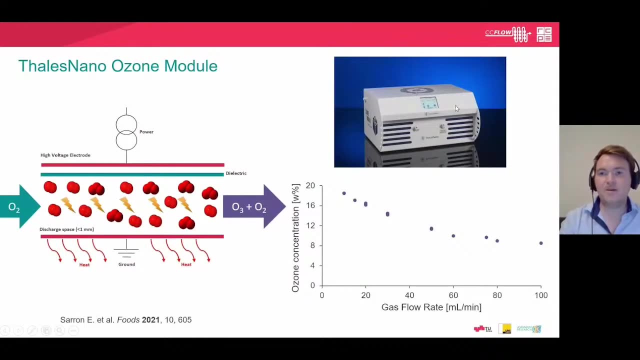 and then one thing that we always did before each experiment is to perform a leak test with an inert gas to ensure that um gas wasn't um, so that the system was sealed um. so in terms of the talis nano um system that we were using, so this can operate between 100. 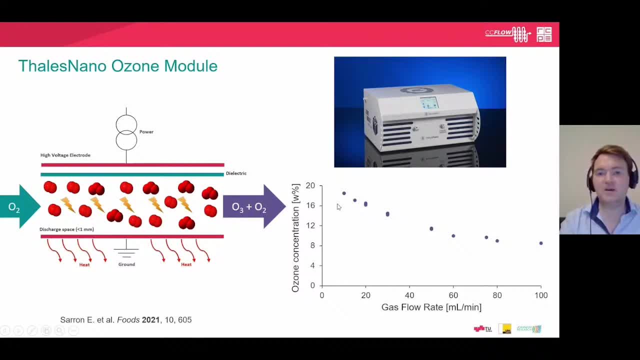 milliliters per minute down to one milliliter per minute, and it can generate ozone concentrations between approximately um 18 weight percent and about um eight to nine weight percent, depending on the flow rate that you're using um, and it can operate up to a pressure of five to six. 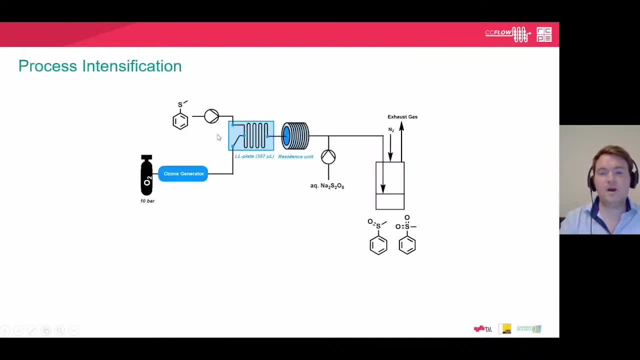 but um. so the first system that we looked at was the um, the ozone analysis of thioanisole, and this can form our desired um product. and then also uh, the over reaction to uh, to our um, to, to to uh side product as well, by using the ozone device. 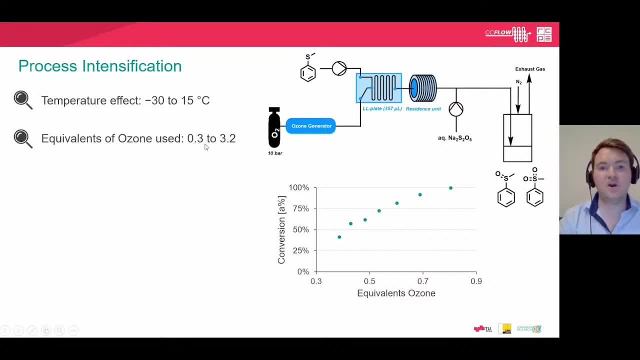 so we looked at a number of different parameters. so we looked at temperature to see the influence that that had. we looked at a wide range of ozone equivalent used, as you can see on the right hand side, um as you would expect, with increase in equivalence, then you have um higher conversions um. one thing that's interesting is, you see, 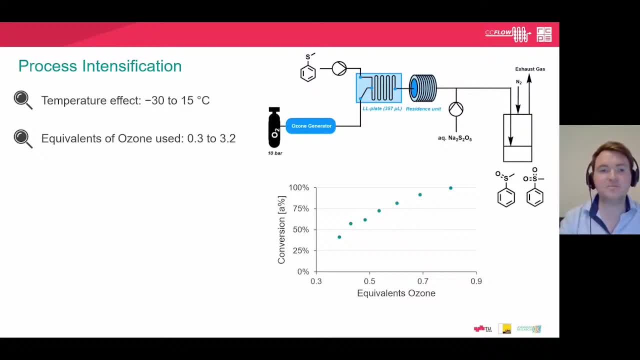 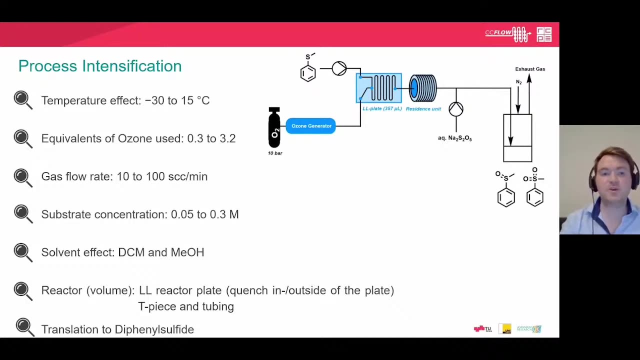 which indicates that it's probably a radical mechanism that's occurring. We also looked at gas flow rates along with liquid flow rates to look at the resonance time that was necessary within the system. We looked at different substrate concentrations. We looked at two different solvents, both dichloromethane and also methanol, And then we also investigated. 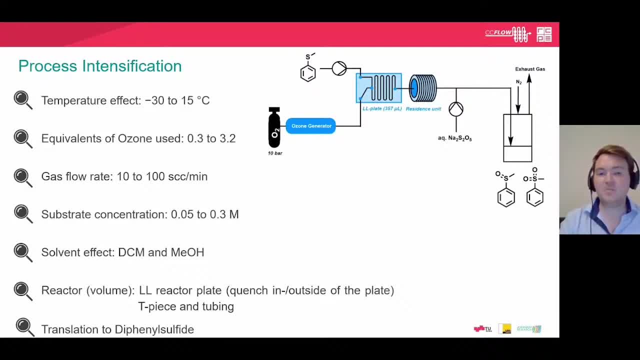 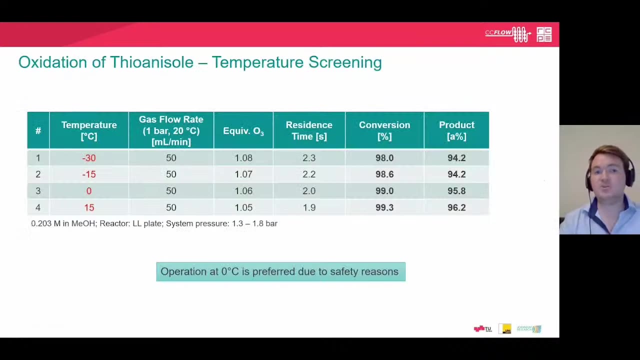 the reaction within a reactor plate and then also just using T-piece and tubing, And we also applied the same conditions that we identified for the ozonolysis of diphenylsulfide. So, in terms of temperature, what's interesting is that temperature doesn't really have an influence. 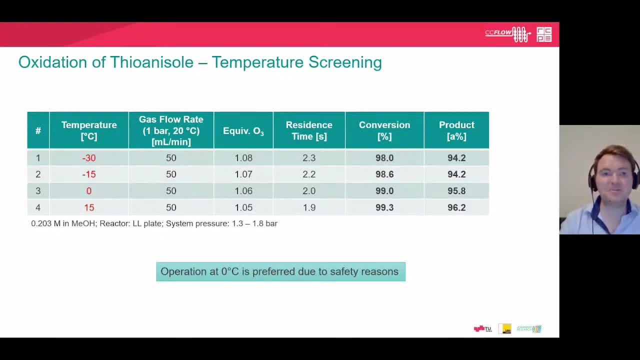 in terms of the reaction performance. So at minus 30, we see 94% Area percent of our product, And then at 15 degrees we see about 96% of our product. So we decided, in terms of our focus, to look at nought degrees Celsius and then also in: 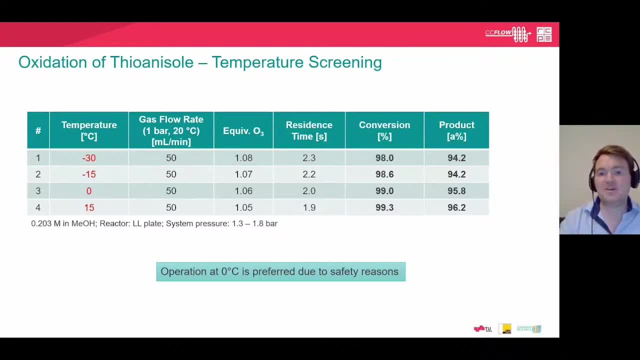 terms of our long run nought degrees Celsius, because then this is operating below the flash point of our solvent, And then, as you can see, here we're only just using a slight excess of ozone and our resonance time is relative The short of only around two seconds. 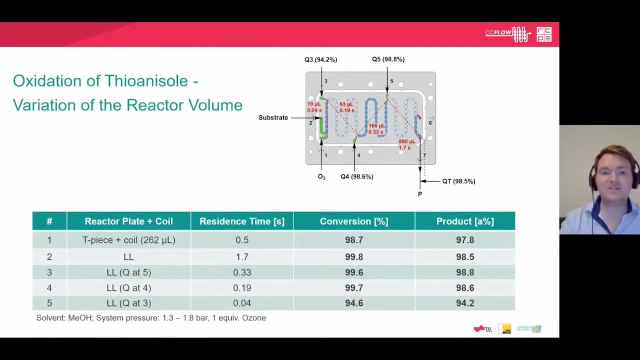 So, looking at the reactor volume and the and the mixing and the influence that that has. So for our first experiment, we just tried it using a simple T-piece and a short coil at half a second resonance time. And what's fantastic is that, as you can see, you see, 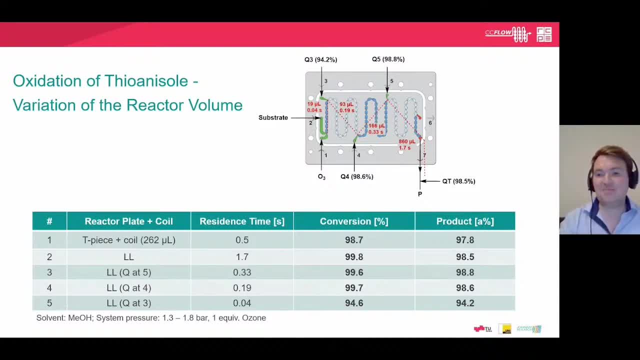 high conversion and high product formation. So the thing that this shows is that clearly at this scale It works very well within a T-piece, And then also when we take the flow plate and we look at different reactor volumes here and different resonance time. 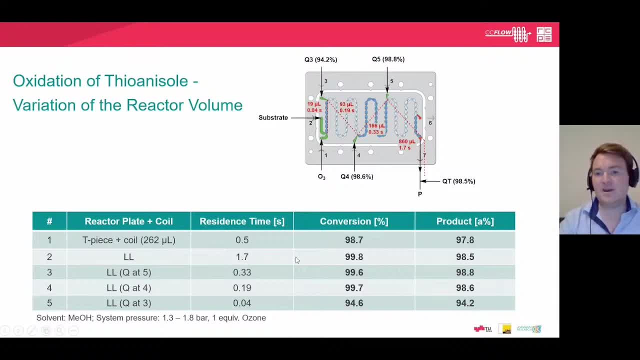 So at 1.7 seconds within the flow plate, then we see very high conversion and then a slightly marginally better area percent for our product. And then as we reduce the reactor volume by using different quench inlets, then you see you also achieve very high conversion and comparable area percent. it's only when we go to 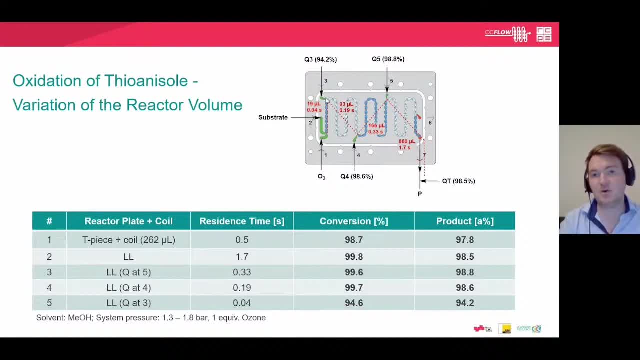 very short residence time, so quenching within the first corner, at q3, within the flow plate, that then we start to see a drop in conversion and product yield, and so it shows that even within a short time, so in terms of scalability, even though at this scale the t-piece and coil perform similar, 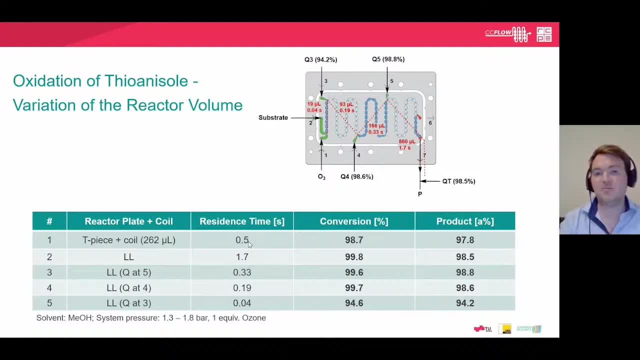 to the flow plate, as if this was to be scaled up. then can the same mixing and thermal management be achieved within a two piece and a coil? and the answer is, uh, probably not so, which is why you would then look to perform it in a, a micro reactor that could give you that, that careful control. 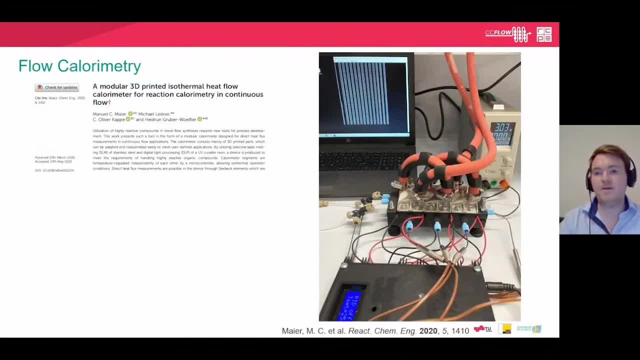 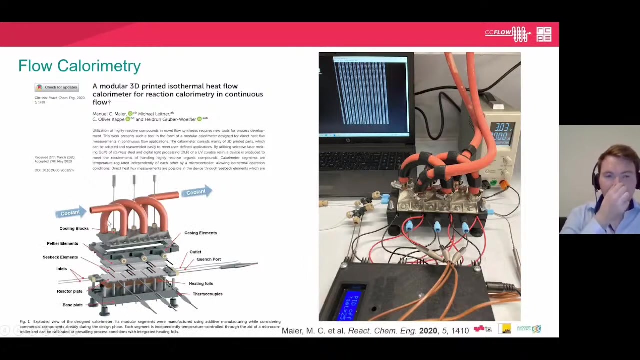 um. so we also looked at the um, the transformation within a heat flow continuous flow calorimeter, which was developed in at tu graphs here. so this is a picture of it on the right, um, so um, and then an exploded um version of it in terms of. so it uses uh peltier elements to um to measure um, the um. 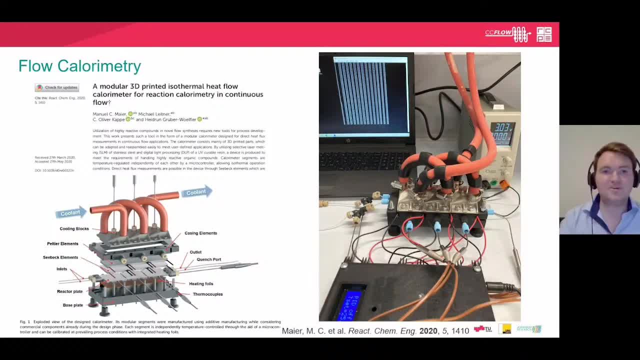 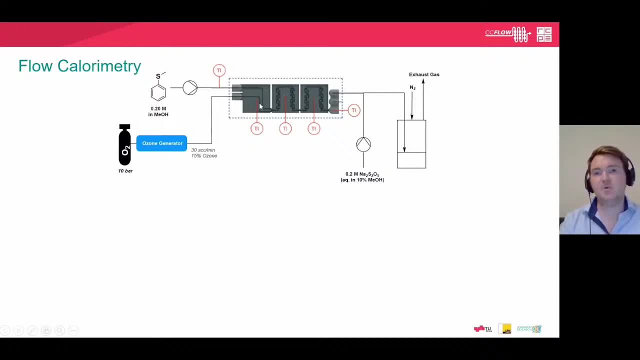 the, the um to to measure the heat of reaction, um. so this is a bit more of a detailed schematic in terms of the way that the segments are set up. so within the first one there's the opportunity to pre um, preheat or pre-cool, and then you have two. 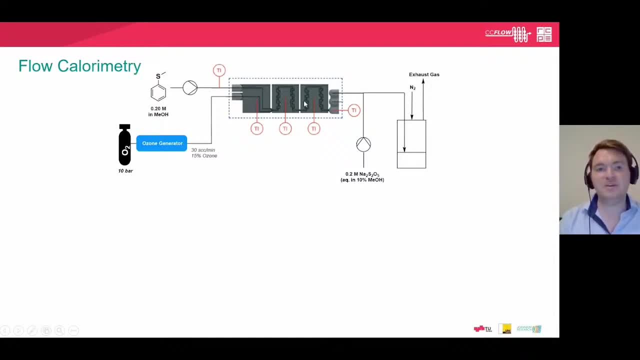 uh, reactor segments, uh, where your two feet are mixed um, so it's a very similar setup to the flow plate, and then within this, then a very good calibration is necessary so that you know that, uh, uh, so you can be confident in the measurements that are taking place. 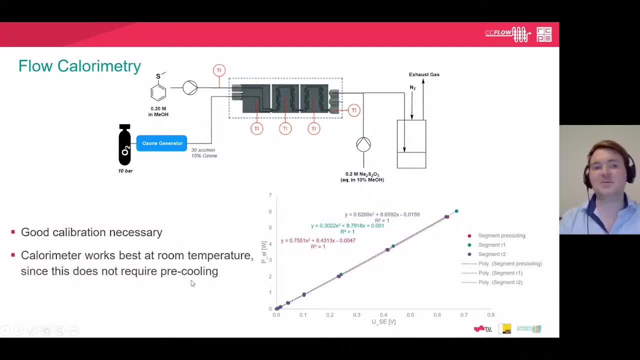 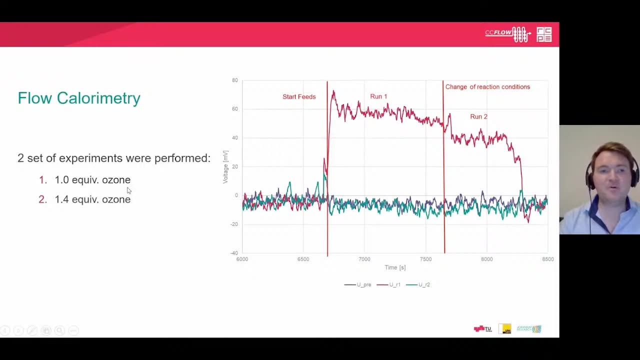 so, as i say, the operating a room temperature has a benefit that then you don't need to pre-cool, so you're it's, it's a lot better in terms of um that, and so this is uh. it just shows the results from two separate uh experiments that were performed, so one equivalent and 1.4 equivalents. 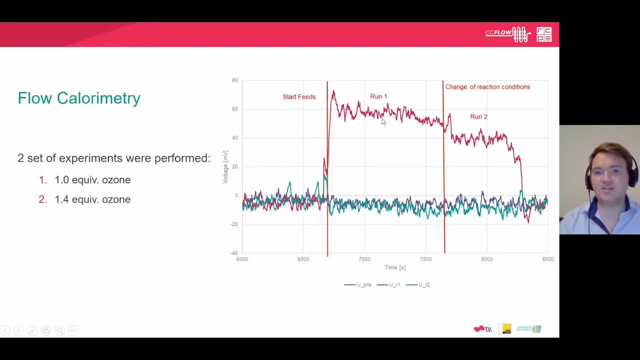 as you can see, uh, this, this shows the change in voltage. uh, uh. so this is the first set, and then here is the second set, and then, based on this, we could quite confidently, uh, measure the heat reaction. so, minus 165 kilojoules per mole, which corresponds to a an adiabatic temperature rise. 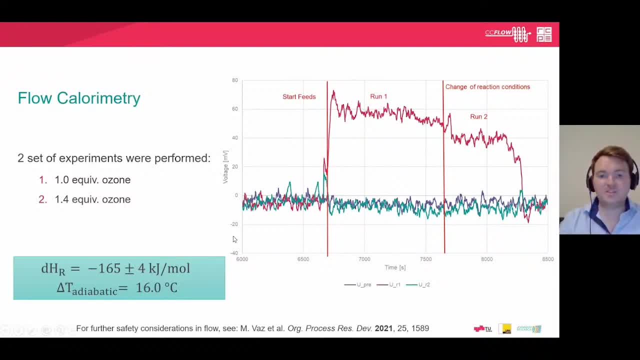 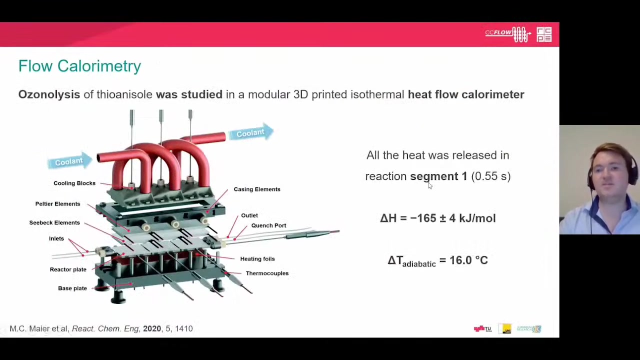 of 16 degrees in terms of considering safety within ozone analysis reactions. i refer people to this great publication from corning where they go through a lot of the different considerations that users should consider. so, yeah, i think the thing that's very interesting within within the calorimetry experiments that 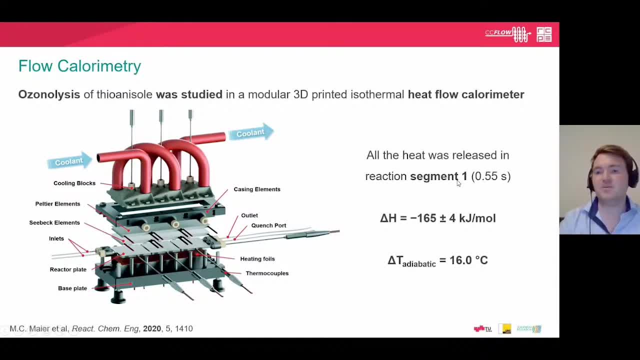 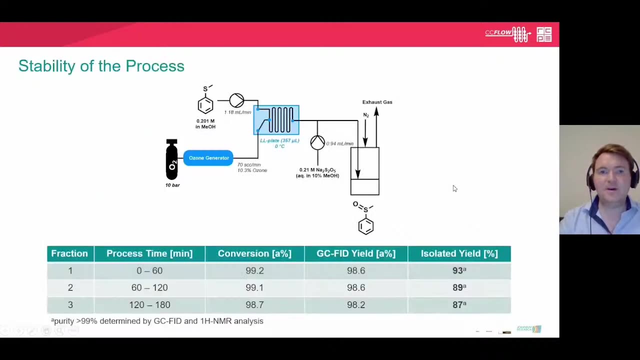 were done is that we saw that all the heat was released within the first segment, which corresponds to a residence time of 0.5 seconds, um. so it happens very quickly and there wasn't any any heat released in the second segment, um, in terms of looking at the stability, we also want to show that not only does it, 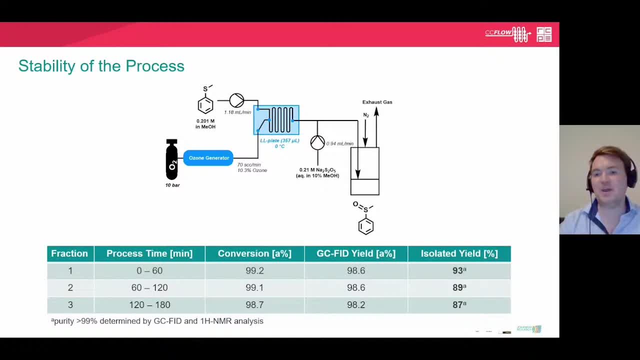 work during our optimization experiments, that that actually we get consistent results as we operate the process for longer and we looked at it over a period of three hours and we saw uh based on the optimum conditions that we were using uh around one milliliter per minute of our um liquid fee, 70 milliliters per minute of our um. 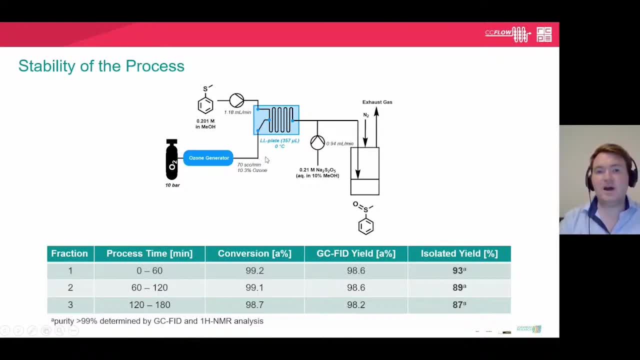 of our um ozone in oxygen gas and within the flow plate. and then then the quench that we saw very good yields in terms of almost quantitative yields and then, after isolation, close to 90 yield. so it shows that it it works for a prolonged period of time. 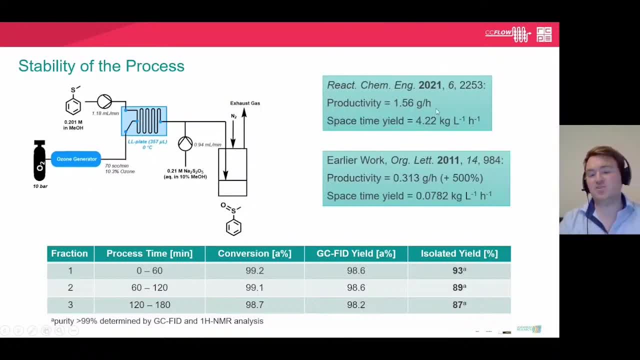 um, and the thing rarely to stress here again, coming back to the space time yield, is that this offers a far better space time yield compared to earlier work that was done within a tubular reactor, and also in terms of the throughput as well. uh, because, because, um. 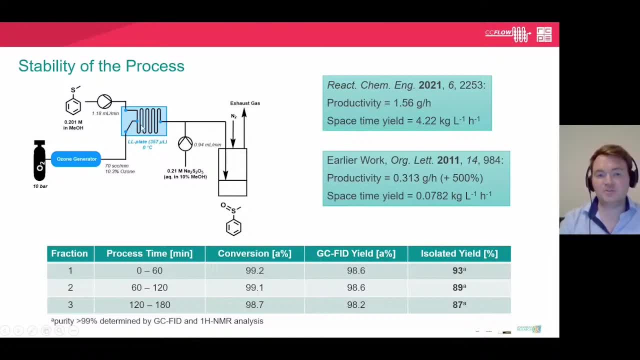 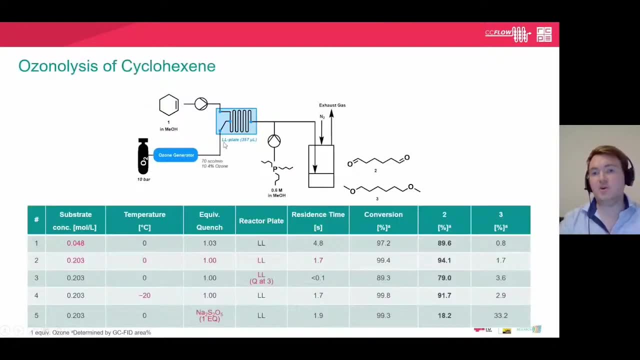 because, uh, quite high because of the short resonance times that can be achieved within the microreactor. so we looked at a slightly different chemistry in terms of the ozonolysis of cyclohexene, using so with similar conditions as for thioanisole. so we looked at a low concentration and 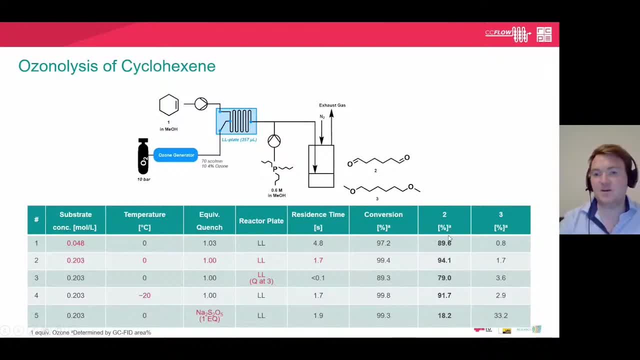 a long resonance time and saw that you could get 90 percent of the desired bisaldehyde, and then even at higher concentrations, um, at a shorter resonance time, then this led to an increase and then, when we had the quench at an earlier inlet, then we saw that they again in a similar 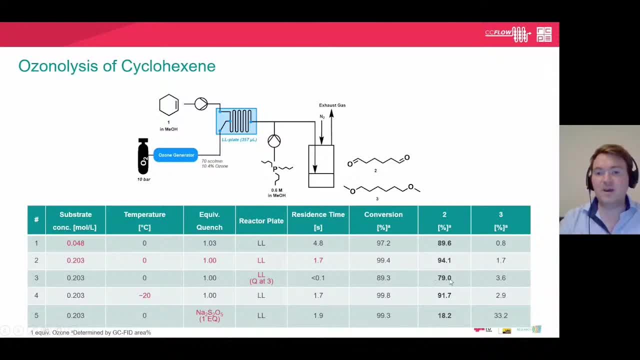 manner to the thioanisole, that there was a drop in conversion and then also a drop in yield as well, and then at lower temperatures, this provided no improvement. so it's great that we can operate this process at zero degrees. and then, when we changed the quench, then we saw that there was a big drop. 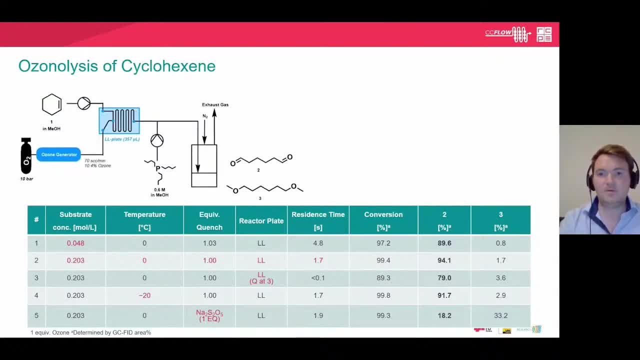 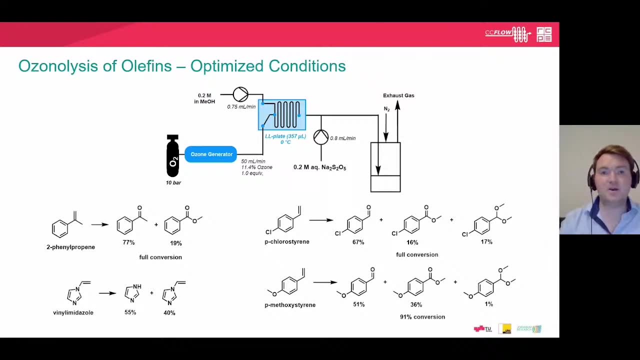 in our desired product, and then we also applied these conditions to look at different substrates, uh, using methanol as well. we also looked at these substrates in dichloromethane as well, whereby we saw a an improvement, um. so, just looking at the methanol example. so, as you can probably imagine, 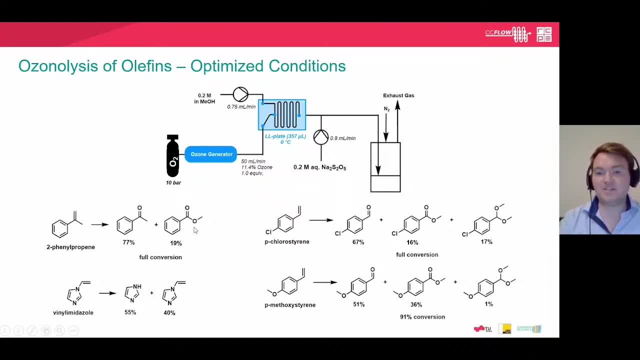 you do see the um, the esters formed for these substrates, and then also um, these substrates, and then also the acetyls as well, um. so it's important that our desired transformation takes place before um, um, the, the reaction with uh methanol. so it needs to be carefully, uh fine-tuned. 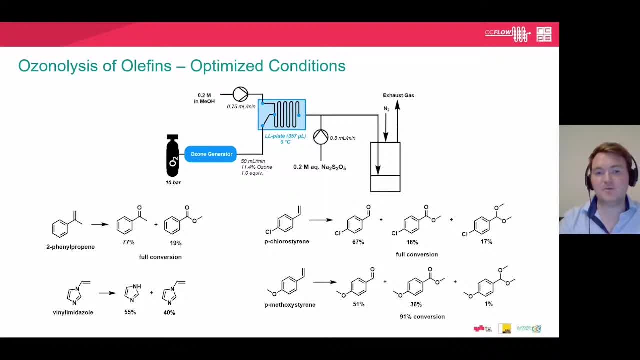 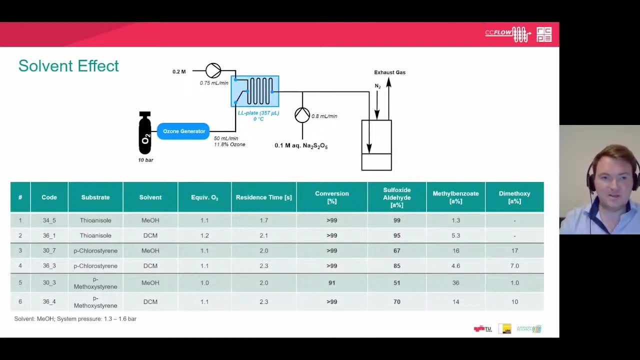 and, as i say, using dichloromethane led to slight improvements with all of these yields as well. but this is not showing um. so here we can see, uh, the improvements that we saw with dichloromethane. uh, so um in here, so with um power chloro styrene. so here, 67 to 85, and then again. 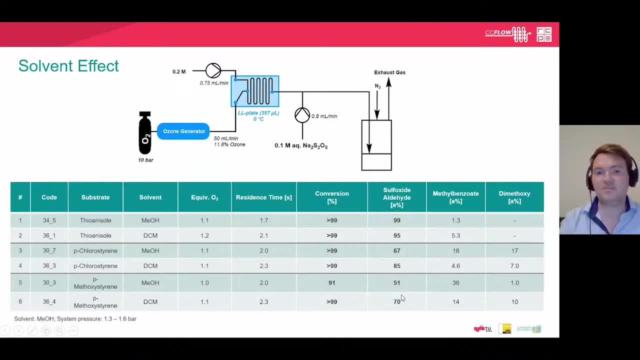 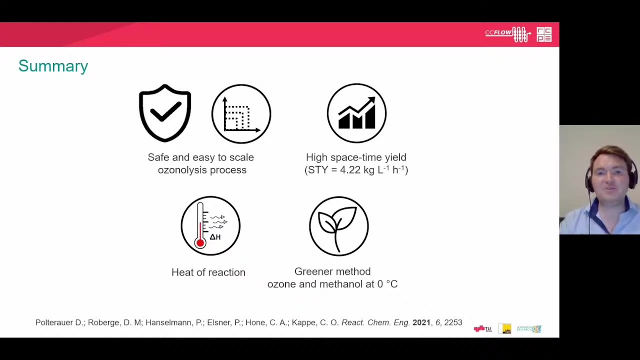 with paramethoxystyrene, again from 50 to 70, so um it could further improve um our desired product. so as a an overview, um so i hope i've shown that uh, we can use continuous flow technologies to safely um operate these types of processes, and also it gives us the opportunity to 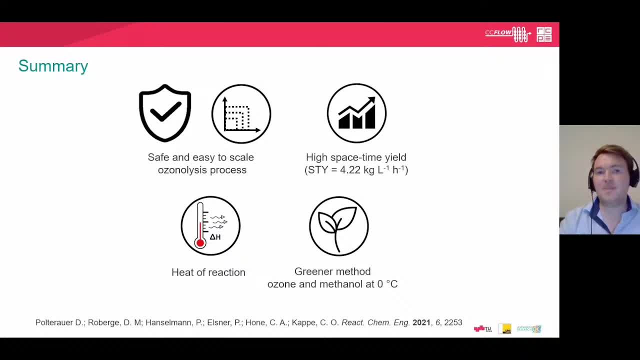 uh to take these processes and uh scale them up. um high space time yields can be achieved uh with this type of uh process because of the short residence times that are possible. i also showed you that we used a 3d printed heat flow continuous flow calorimeter from our 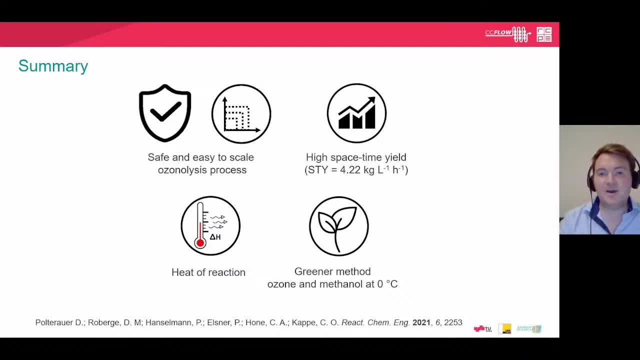 colleagues at tu graphs to measure the heat of reaction uh for these um for this type of transformation, and also in terms of the, the benefit that methanol might have over dichloromethane in terms of providing a greener method, as we saw with the last examples that dichloromethane can. 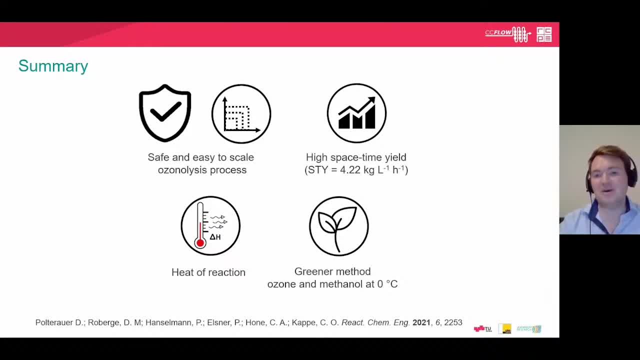 sometimes give us a better yield, depending on what product we're after. actually, if we can use methanol instead and fine tune towards that, then that might lead to an improvement. so you can read about the research that i presented within this webinar in the paper that's at the bottom. 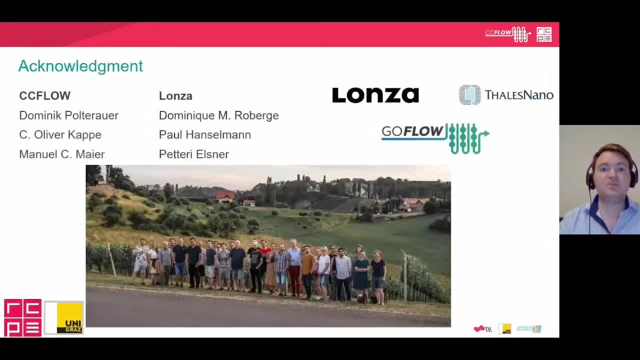 and there's more details there as well. so i just would like to acknowledge my colleagues, both at cc flow- so dominic did the lab work, so he worked hard on that- and performing the analysis as well, My boss and the group leader, Oliver Capper, and also Manuel Meyer for his support with the calorimetry experiments. I'd also like to thank 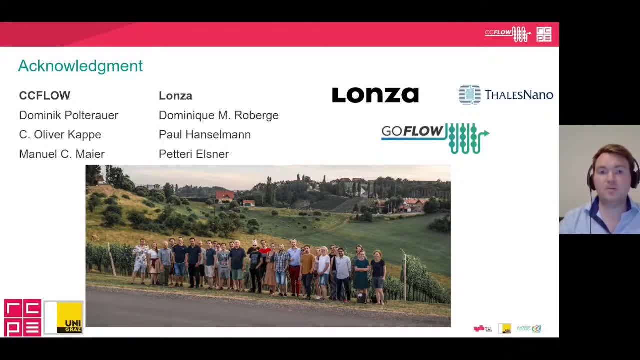 Dominique Paul and Petteri from Lonza for their support throughout the project studying the ozone analysis reactions, and then also, I'd like to thank Thales Nano as well for the opportunity to present the work today and to give this webinar. So thank you very much and I'm more than happy to take any questions. 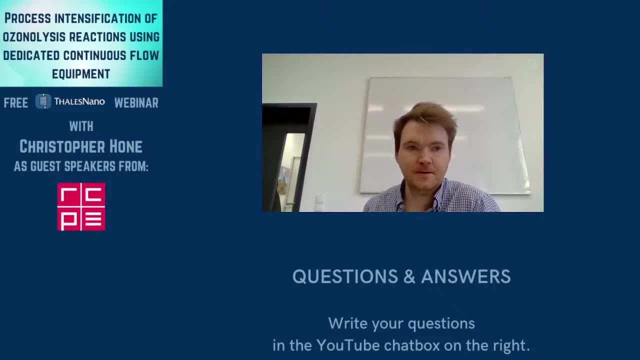 Thank you, Hi, everyone. so now I'm here to answer any questions that you might have from the presentation, So So please feel free to write them into the chat. So if I can't answer them, then what I'll do is I'll be able to contact you at a later date. 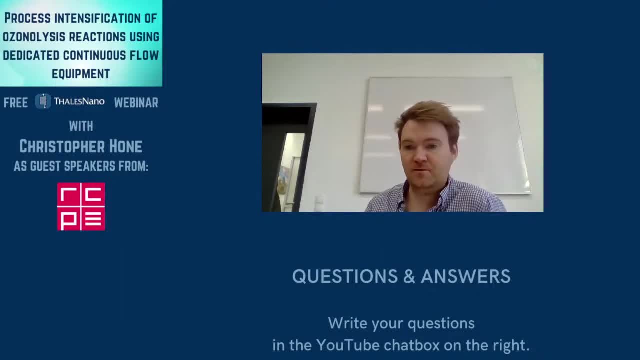 So I'm sure you can contact me via my email or, if you get in touch with Tylos Nano, they can send the questions to me. So, yeah, please feel free to ask anything regarding the talk. So I see one question that's already in the chat, which is about the quenching of the ozone ion for media with hydrogen peroxide and the mechanism associated with that. 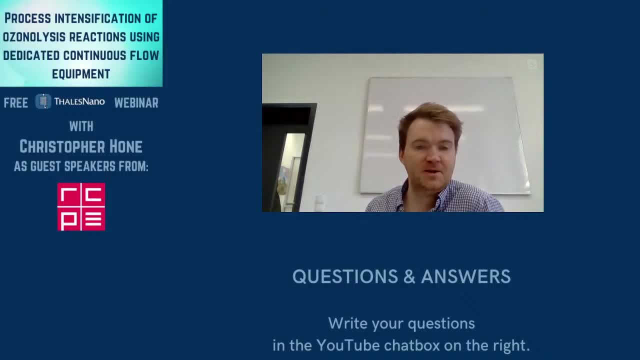 So I'm not sure exactly how much work has been done specifically with hydrogen peroxide and the specifics to the mechanism. So in this case, so when you normally You get an aldehyde and you get a carboxylic acid, assuming that you have a CH on your alkene molecule- 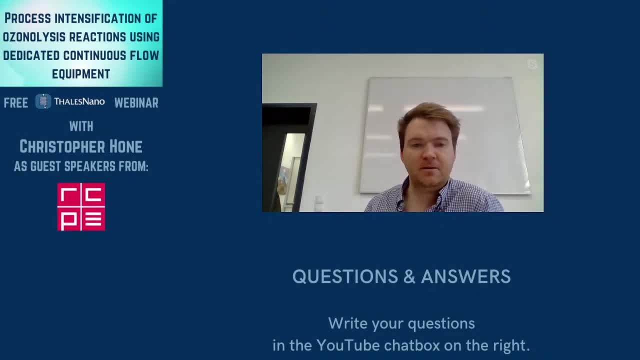 But in terms of how that reacts with the intermediate, I'm not entirely sure. So what I'll do is I'll look into the literature and I'll be able to provide more information on that to see how much has been demonstrated. Thank you. 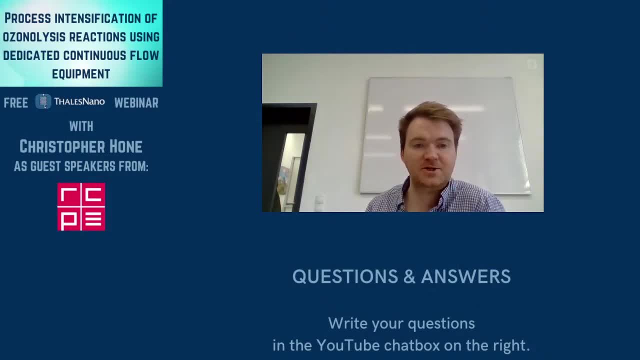 So I'll go through any experimental studies or computational type studies. Yeah, So another question that I got sent as well was in terms of- Let me just have a look- Was in terms of using tea pieces. So I think what was interesting in our studies is we did. 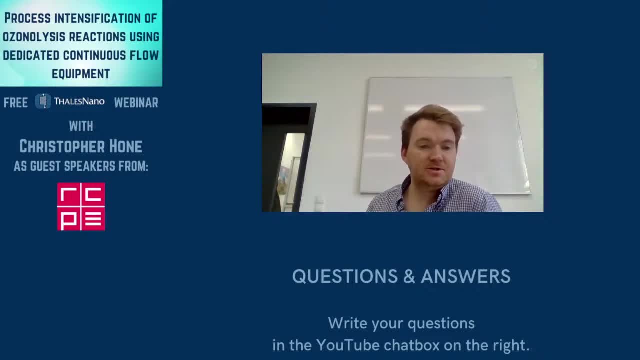 We did a comparison between a tea piece and the float plate, with the specific geometry in the mixing, And we saw quite similar results between the two. I think in some ways this is good, because if you're operating at a small scale, it shows that a tea piece with a small bit of tubing afterwards is fit for purpose. 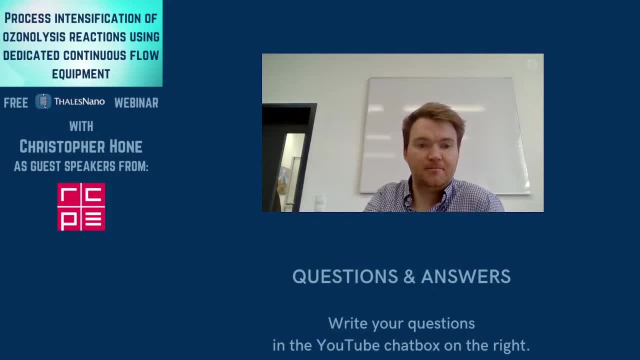 I think the thing is: is that then What you'll find as you go to larger scales? is that then the tea piece can't be scaled to provide the best performance because of heat transfer and mass transfer effects, Because it's not possible to achieve the same as you approach large channel dimensions. 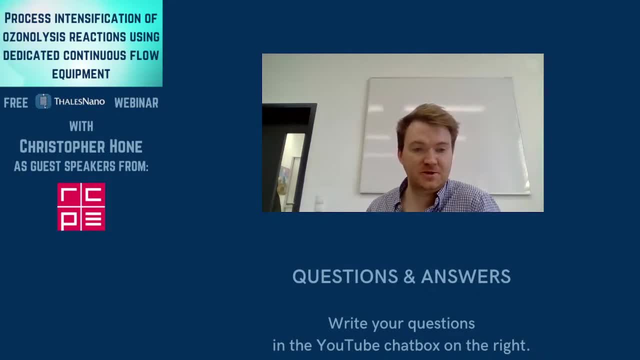 And this is where you start to perhaps see a difference, because it's Because the heat management is harder to Control and, in terms of the mixing, it's harder to To To see, And also in terms of the fact that one thing we like to talk about is something called smart dimensioning. 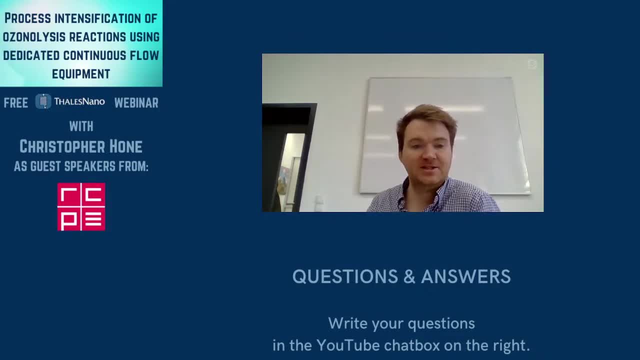 In terms of what you want to do is try and achieve the same heat and mass transfer through careful design of the flow reactor in terms of the geometry, In terms of The channel dimensions and in terms of the same mixing and heat transfer can be achieved at a larger scale than as was observed at the smaller scale. 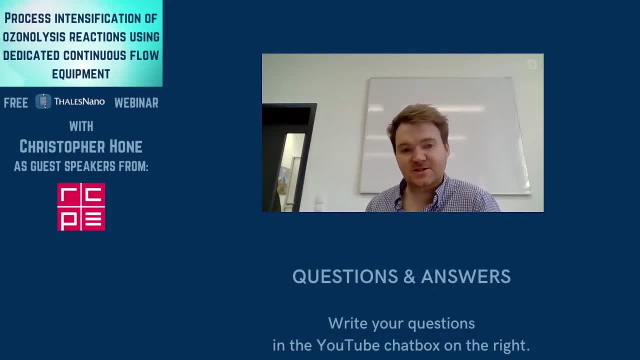 Yeah. So I think this is the interesting thing to know is it's nice that the results are the same, but to scale them you might see differences, Especially with the tea piece. So I've got another question from Phil And he's asking: has there ever been ocean analysis which has looked at the over-oxidation from the thioether to the sulfone? 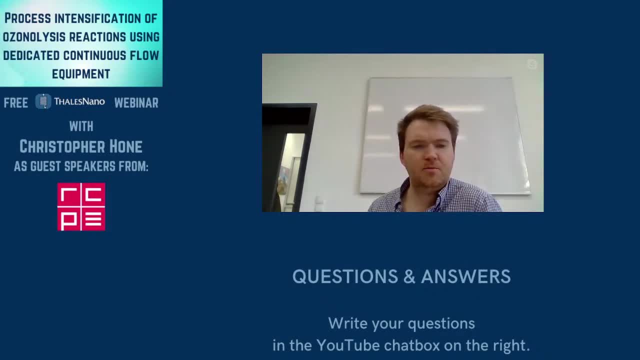 I'm not sure, to be honest. I think that would be quite an interesting thing to look for. I think, in principle, it should be very It should be easy to do in terms of just letting it be, In terms of just using. 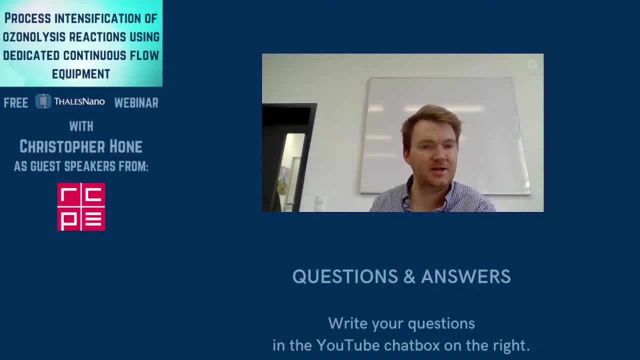 Just by modifying the conditions, because clearly we see it so it's possible. So, whether or not, by using a longer reaction time and no equivalence of ozone, then it would be possible to fine-tune the selectivity towards the sulfone rather than the 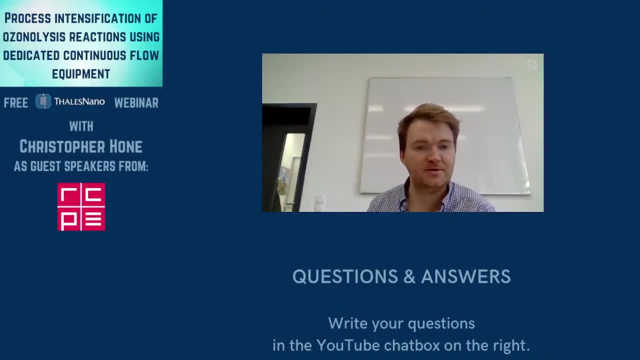 Rather to our desire. The sulfoxide: The sulfoxide, Yeah, that would be interesting to check and look, because then you have the opportunity to carefully modify the conditions to achieve either product. In terms of other questions, Yeah, I've also got one. with regards to the different reactants, 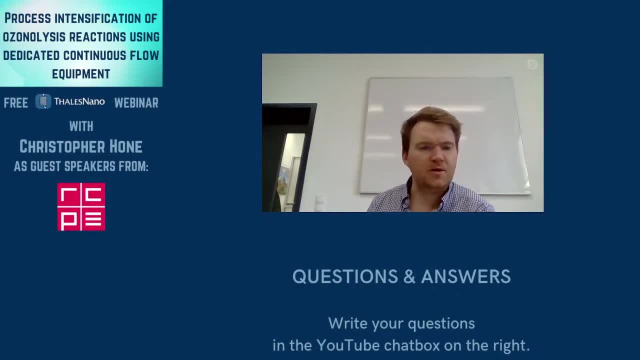 Yeah, The different reactions that are possible and what the limitations are. I had one slide where I talked a lot about this in terms of it's quite a big area of interest, especially in recent years, in terms of those analysis and the different reactors that can be used. 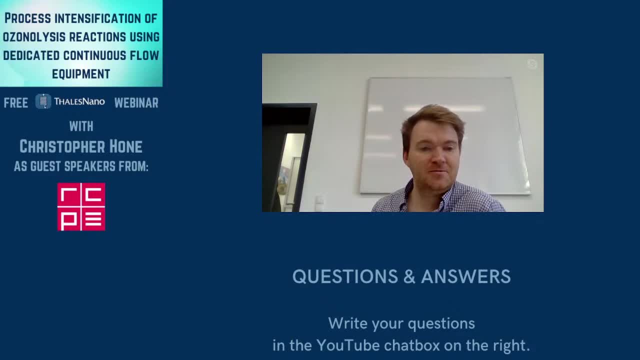 As I showed, there are a number that have been applied. A lot of them are only really appropriate for lab scale and there's not really any scale-up option there, So it needs to be done with care. Clearly, the benefit of operating in flow is the ability to use higher concentrations. 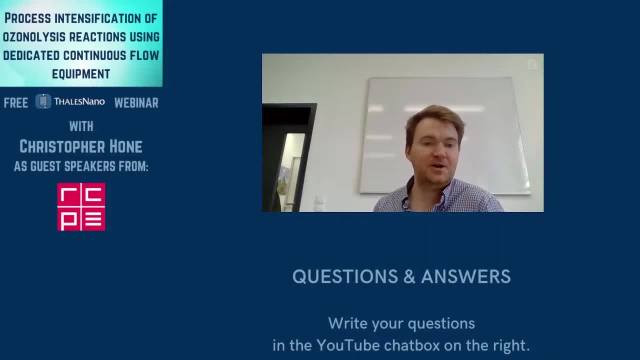 both of the ozone and then also of the oxygen gas in a safe manner. You do have to be careful when using these things, especially in batch reactors and the CSTR reactors as well, because of the headspace and having high concentrations. Yeah, 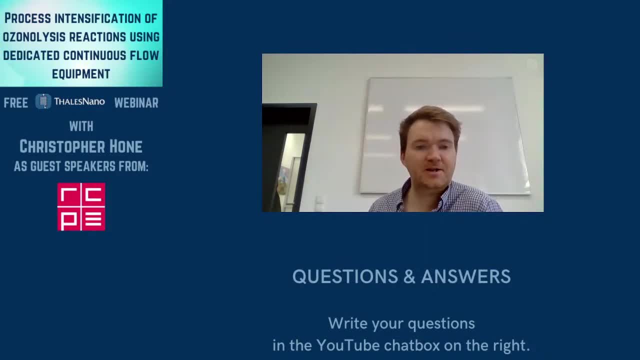 Of ozone, in particular in the liquid phase. Yeah, In terms of the others, I would say, in terms of scalability, then the micro-reactor is the best. There are clearly ways you can do parallelization of the units, but this is only scalable to a certain extent. 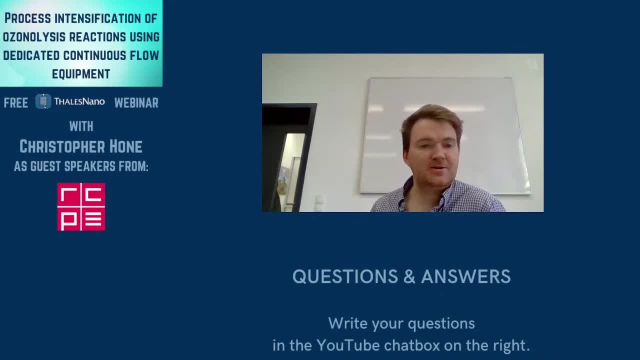 And then you have to apply this principle that I talked about a bit earlier in terms of smart dimensioning The other reactors that I talked about, say the tubing tube reactor. this is very nice, particularly at a lab scale, to be able to handle the gas safely.